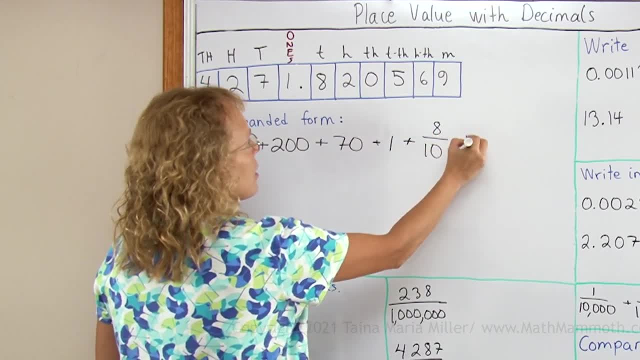 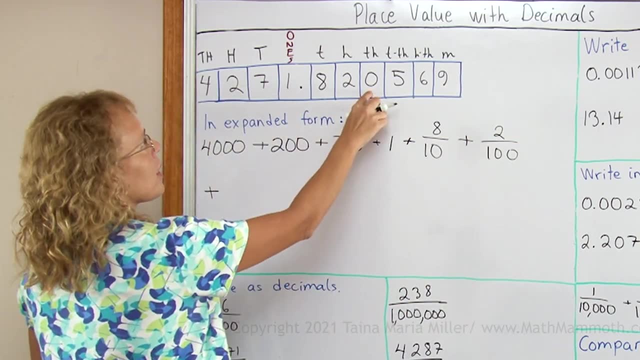 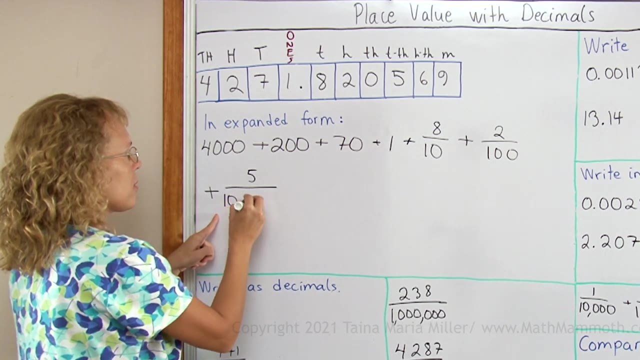 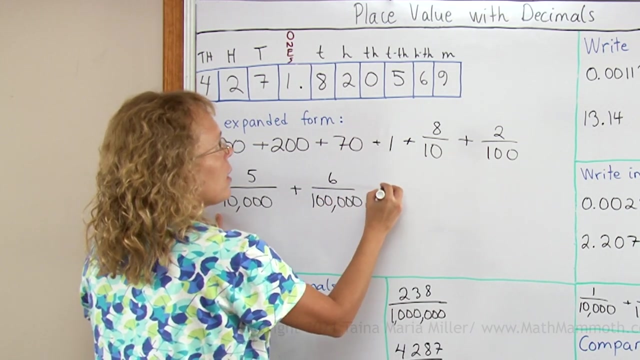 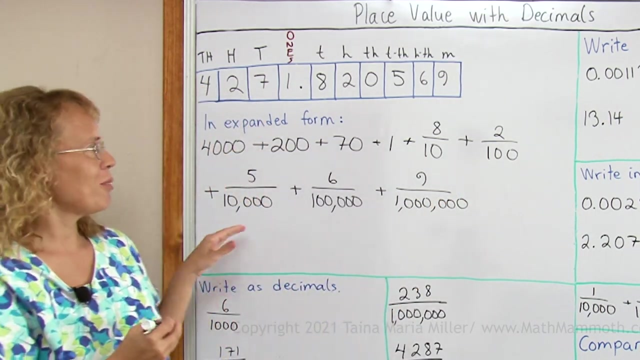 tenths, Next comes two hundredths And next zero thousandths- I don't have to write that- Then five, ten thousandths And then six hundred thousandths and lastly nine millionths. So it takes quite some time to write it in expanded form. 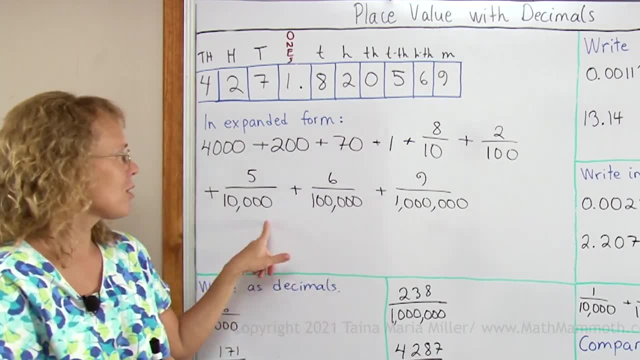 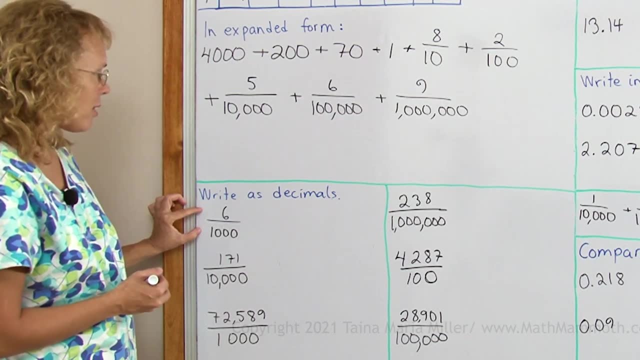 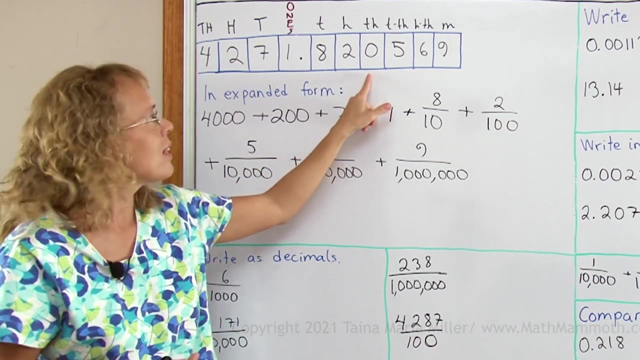 You could also write it in expanded form, using here decimals instead of fractions. Now let's write these as decimals, and I want to show you a little shortcut. Six thousandths as a decimal. Okay, if you notice here, whenever a decimal has thousandths, then it must have three decimal. 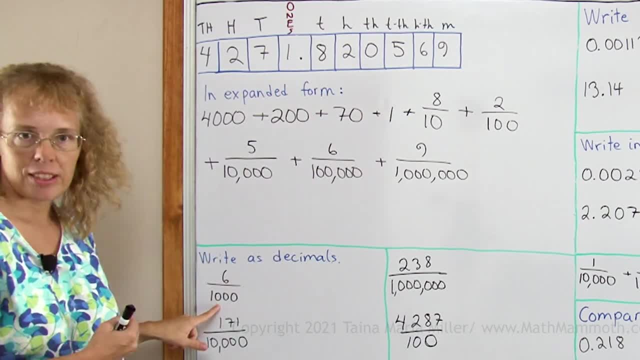 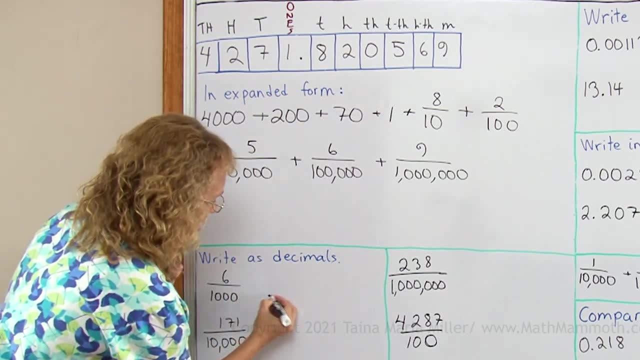 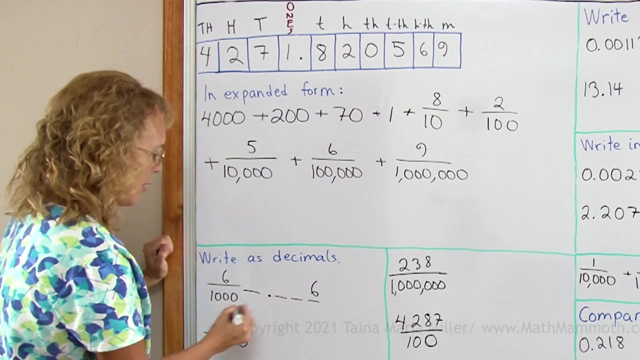 digits. Okay, Just like the number thousand here has three zeros, then we have three decimal digits. So all I need to do is write a decimal that has three decimal digits after the point and put six there here at the last. So now I just put zeros in, so it is zero point zero, zero six. 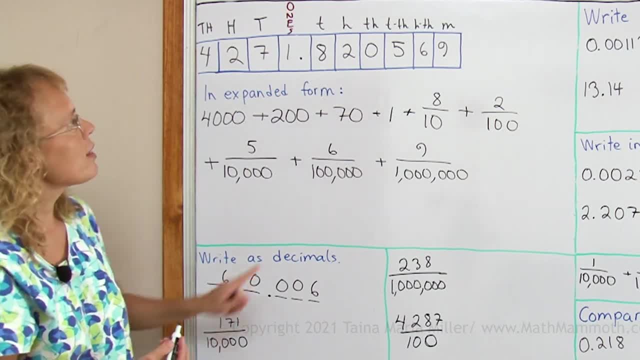 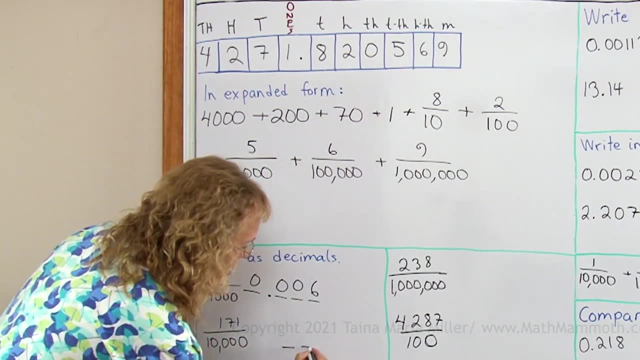 This one here has ten thousandths. Ten thousandths as a denominator, So ten thousandths. okay, it means I need to have four decimal digits, Just like here are four zeros, So four decimal digits after the point, and then I put the one seven and one over here. 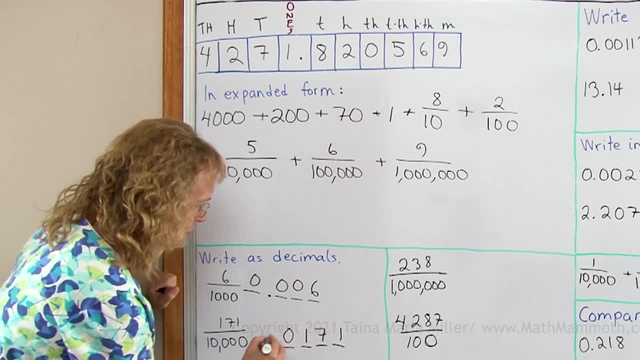 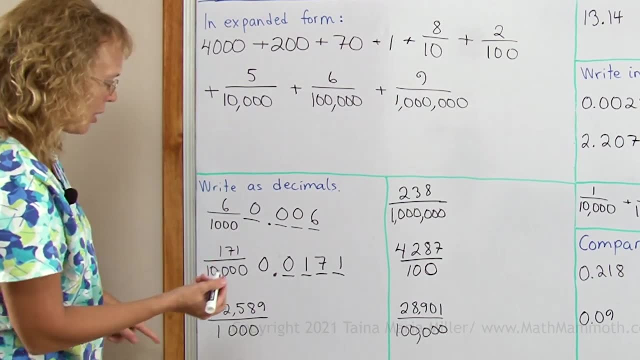 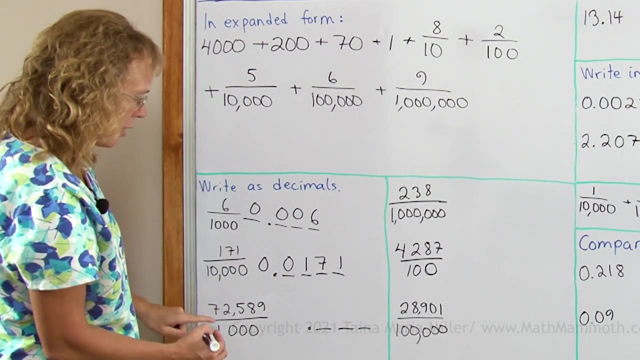 so that something reaches the ten thousandths place, Like that Over here. seventy two thousand five hundred and eighty nine thousandths. The same principle applies here- is thousand, Three zeros, so three decimal digits. But now of course this doesn't just fit there, but it will have seventy two here and then. 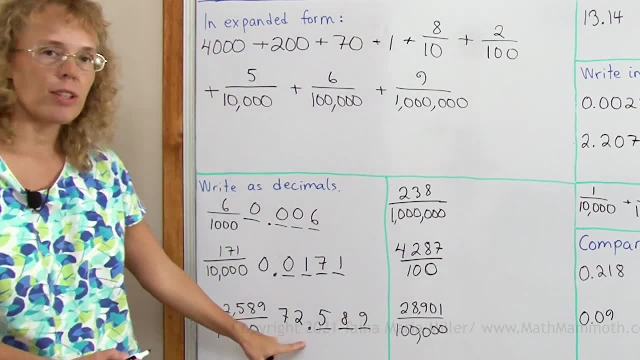 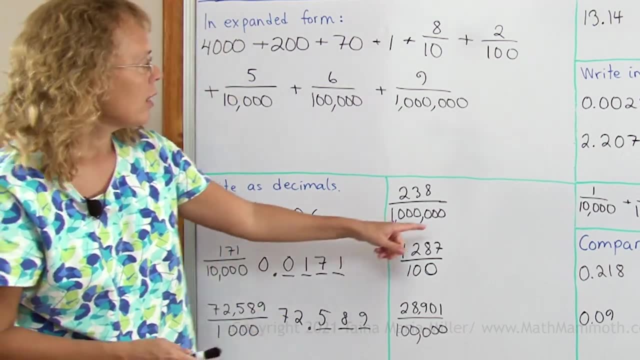 five, eight nine, like that. Seventy two point five, eight nine, Or actually it is the whole number seventy two and five hundred and eighty nine thousandths. Okay, let's try it here. Here's millionths, Six zeros, Six decimal digits. 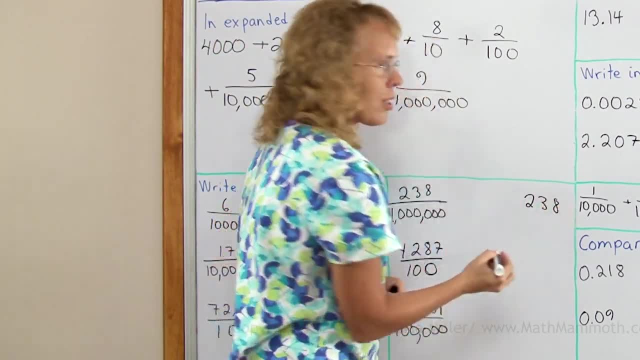 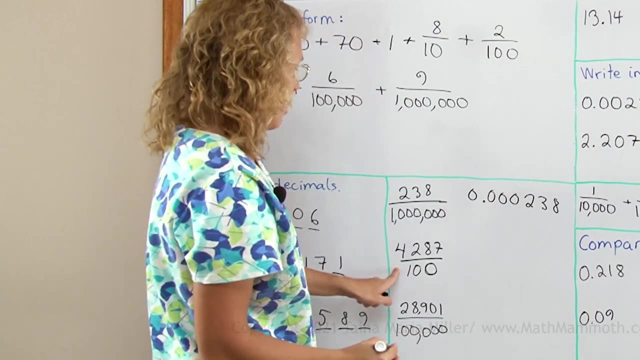 Okay, So two, three, eight goes there at the very end, And then I need to have six decimal digits. Okay, So let's put three zeros here. Then my point Over here: hundredths: Four thousand two hundred eighty seven divided by hundred, or four thousand two hundred eighty. 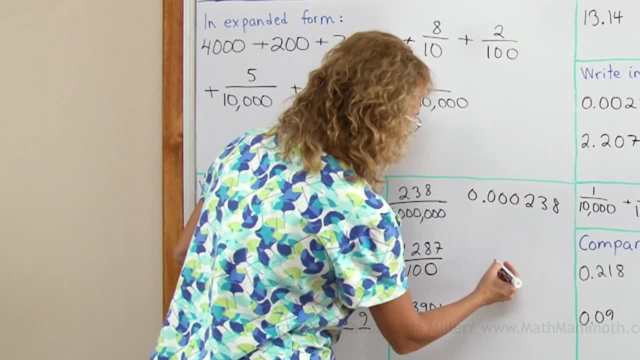 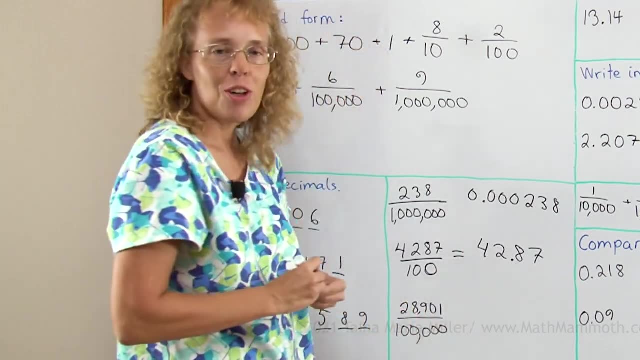 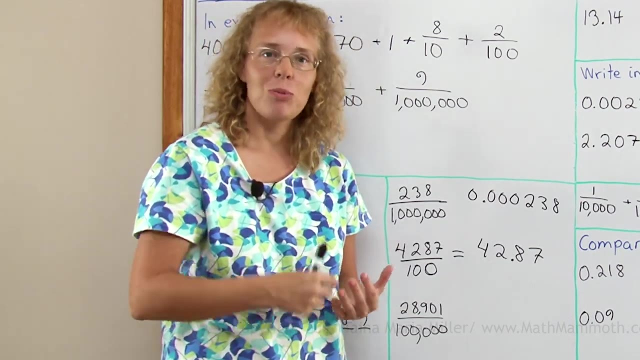 seven hundredths, So I need to have two decimal digits. Okay, I just copy this here and put my point there. Of course, you can recognize this as a division problem too. Four thousand two hundred eighty seven divided by hundred, and the shortcut for that is to: 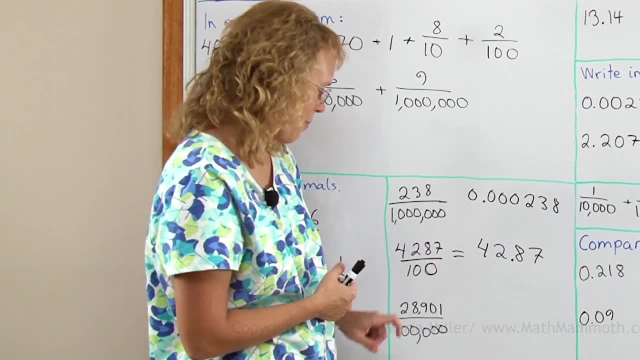 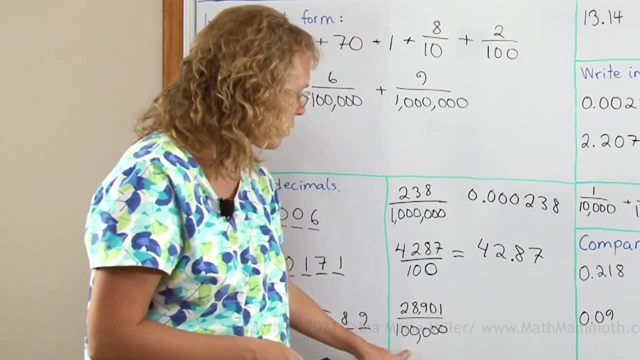 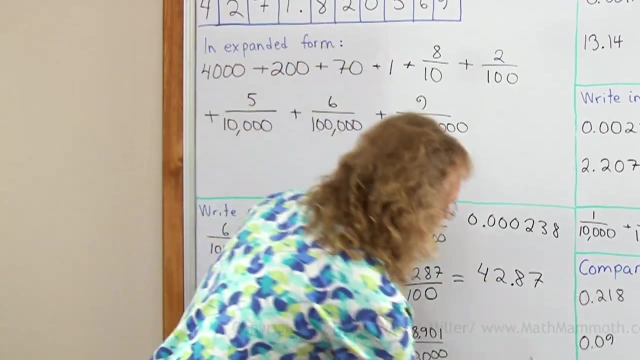 move the decimal point From here two steps over here. Now twenty eight thousand nine hundred and one hundred thousandths. Okay, You see five zeros here, Five decimal digits. Or you can count here One, two, three, four, five decimal digits, Four hundred thousandths. 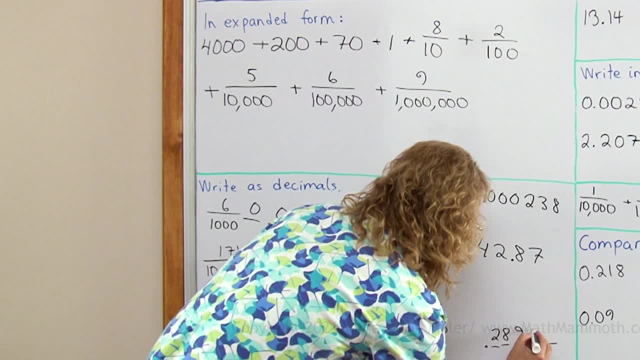 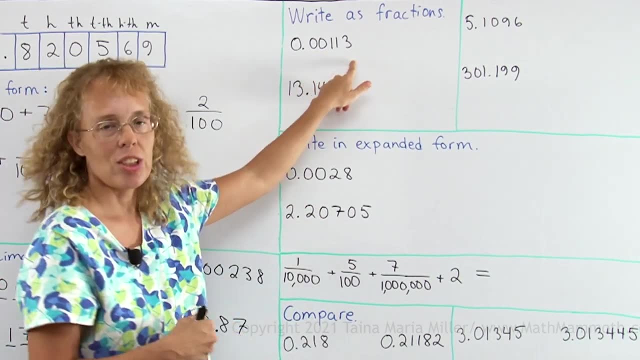 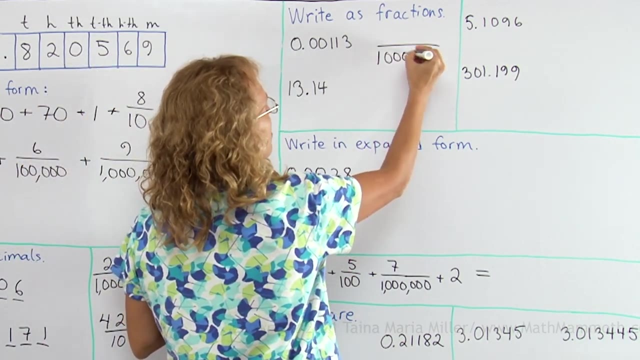 Okay, And my number just goes here Like that: Write as fractions. We will now use the same technique. I'll check how many decimal digits are there: One, two, three, four, five decimal digits. So my denominator has to have one and five zeros. 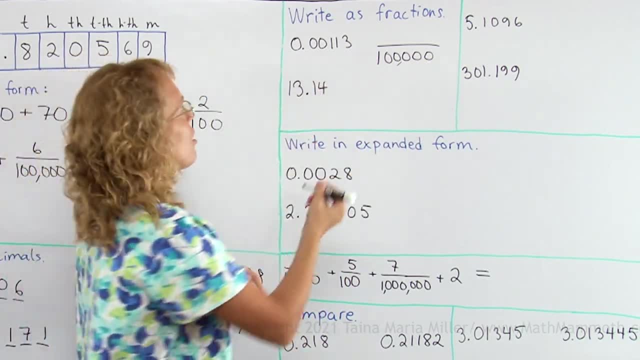 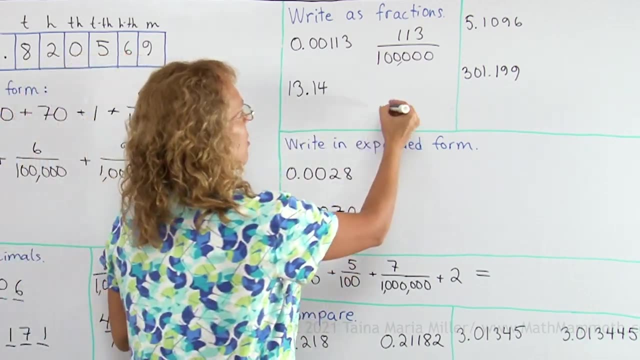 So it is hundred thousand, And then I just copy this number, Those digits here, One, one and three, Thirteen point one, four, Two decimal digits, So the denominator has to be hundred, Right, And then just copy all the digits on top. 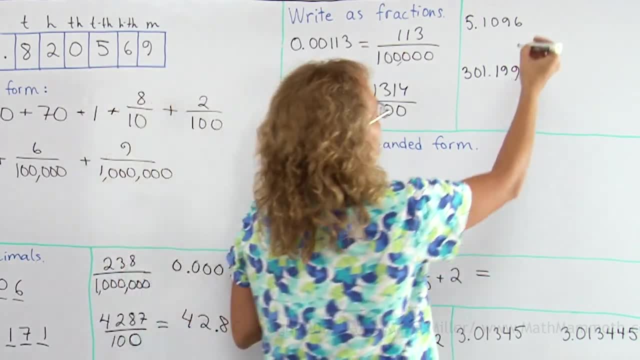 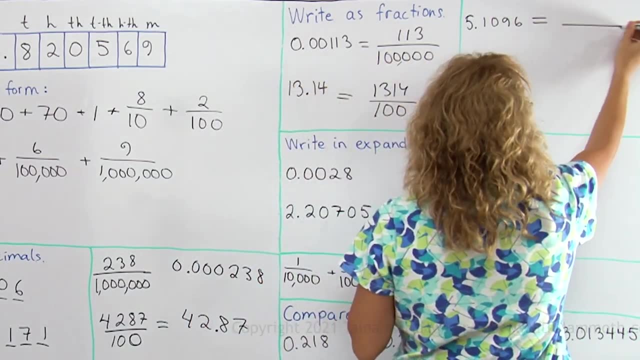 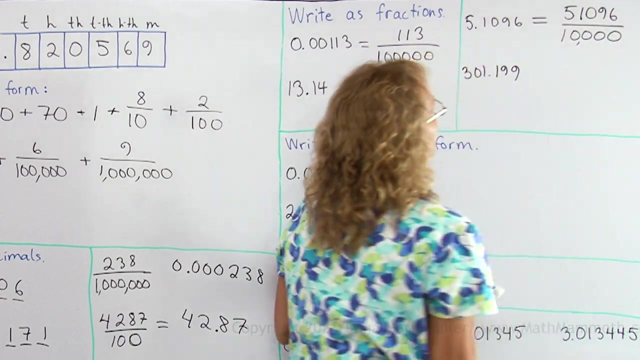 It's very easy Here: Four decimal digits. So what is our denominator? Have to have four zeros here, And then I just copy everything from here, All the digits. So it is fifty one thousand ninety six Divided by ten thousand. 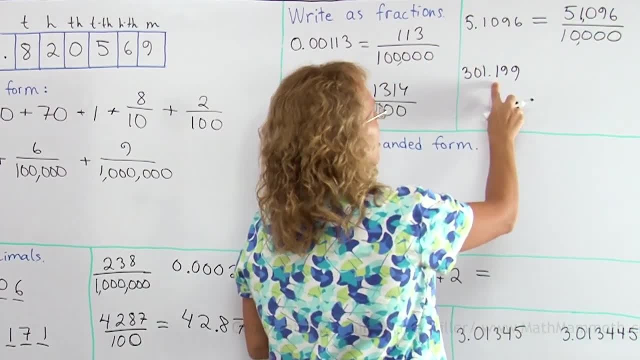 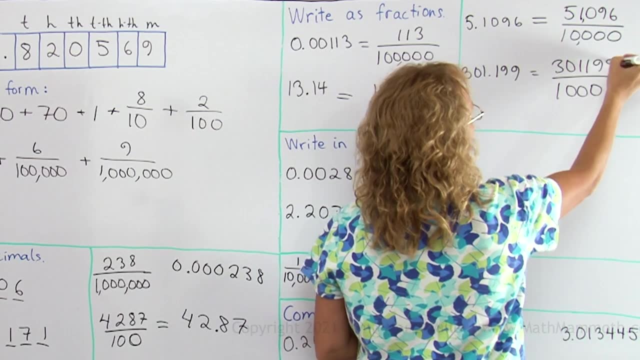 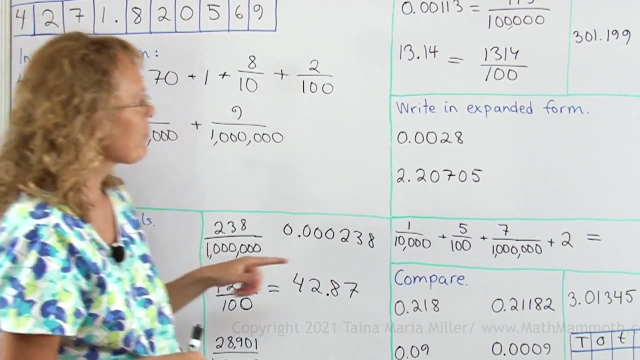 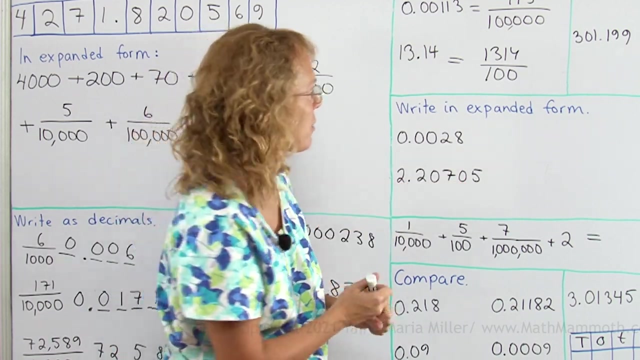 And here Three decimal digits Would mean denominator of thousand, And then just copy those digits over there Right in expanded form, Just like I did here. Okay, This one has two in thousandths place, Right Two thousandths, And then eight is in the ten thousandths place. 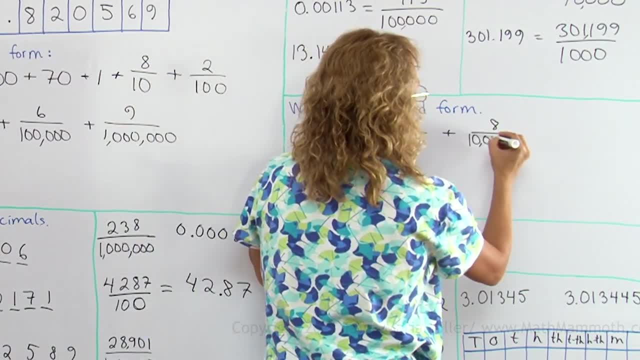 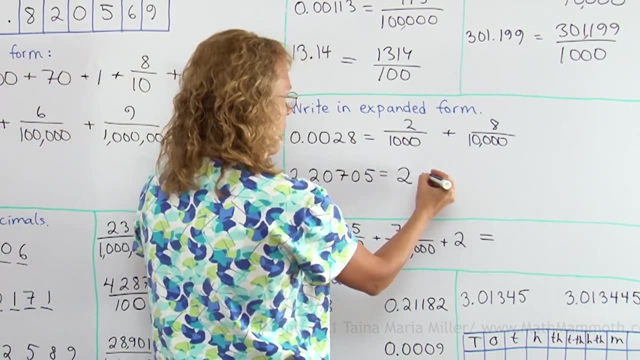 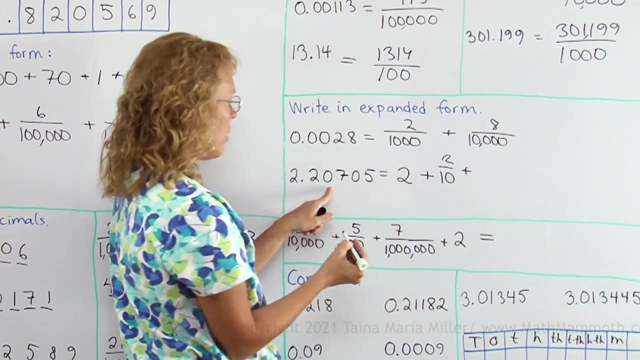 So eight, Ten thousandths, And that's it Now for this number. I will start with this two, Which is just the whole number Two, And then two in tenths place. So two tenths, Nothing here. And then seven is in what place?